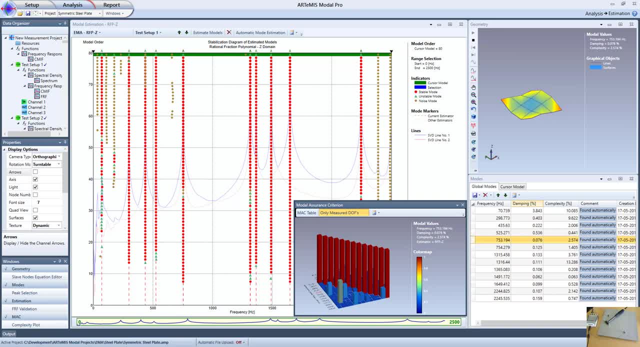 I'd like to show you the latest development we have made in experimental model analysis in Artemis Model. What I'd like to show in this demonstration here is the first part of a test, And I'd like to show how we can do impact testing of a plate like this. 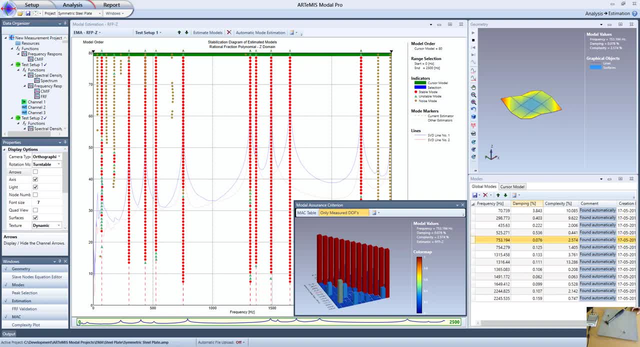 This is a symmetric steel plate, so it has some nice closed space modes. As you can see, I have already connected two reference sensors here, accelerometers, And they are, together with the impact hammer, connected into the national instrument, that data acquisition board we have located here. 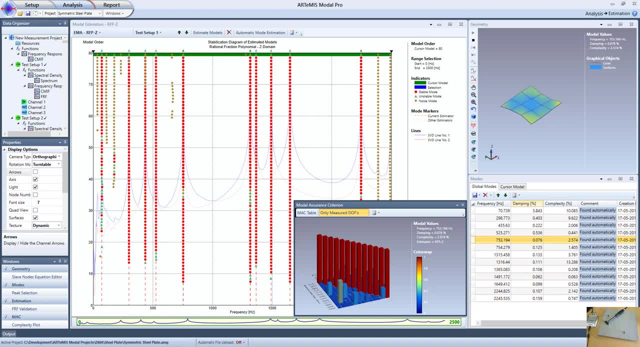 This will then be controlled by Artemis Model in our new impact testing module. So what you can see on the screen is actually the test, how it looks After we have completed it, And I'd like to, of course, repeat this from scratch and show you how to do it. 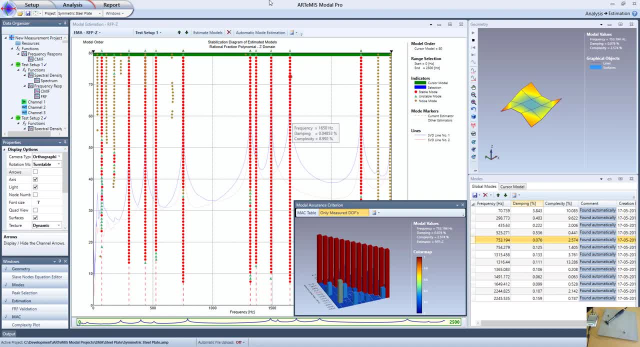 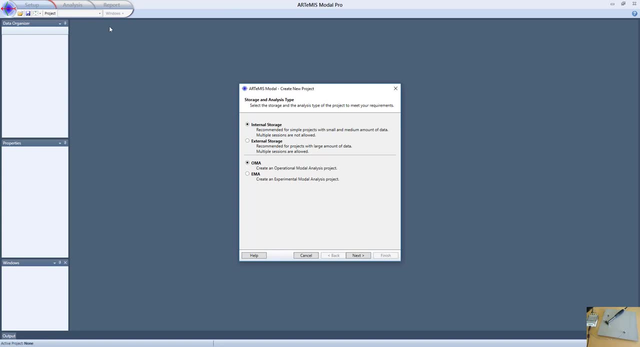 So what I do now is I close this project here and then I will start all over again. So let's start by closing this And then I go to create a new project, And from here we have some different options. What I have to do is I have to inform. 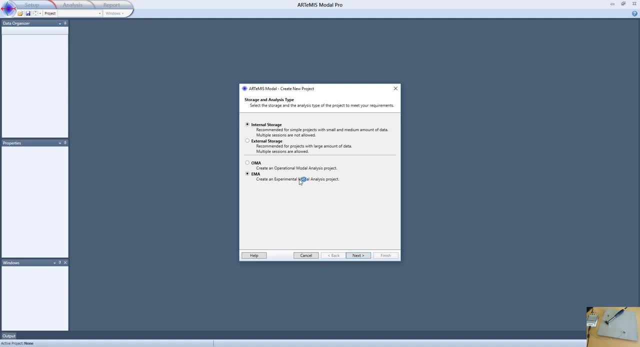 Artemis that it's an experimental mode analysis project that I will be doing. That means input-output mode analysis, And that's actually what I need to select from this dialog here. The next thing I have to specify is then: is it a blank project or is it coming from universal file format? 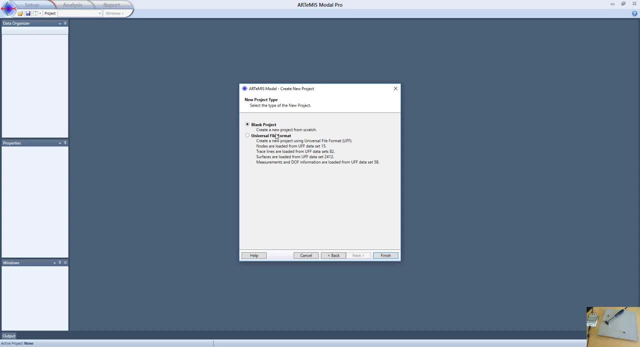 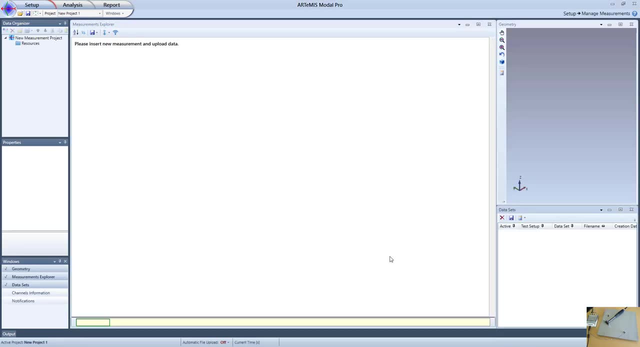 In our case, we will start with this blank project here and create everything from scratch. So I click finish And now I get into one of the setup tasks. It's called manage measurements, But we will jump directly to the first one: prepare geometry. 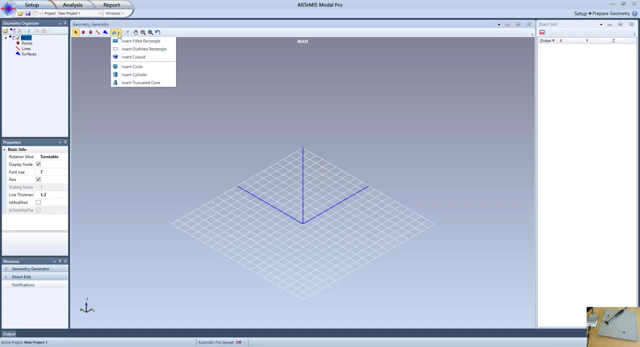 And here we will then insert a predefined rectangle object that can then model this plate here. So I select this one here and then I go to one of the corners here And then I will then go all the way out here to The other corner, like this: 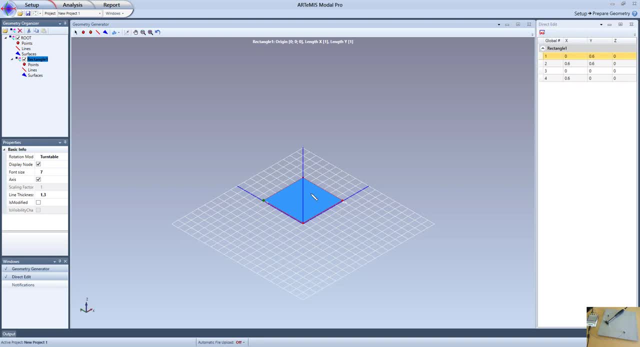 And then I will click, release the mouse button and I have then the plate. Now I have to subdivide this one. here I intend to impact four times along the X and the Y axis, So in total I need to have 16 points available for this. 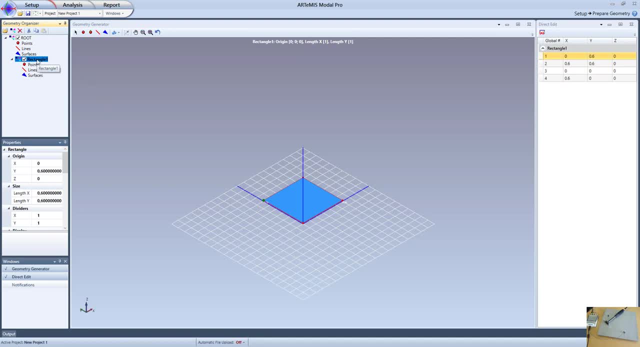 So I click this, Activate this object here, And then I select that I would like to divide three times in X and the same in the Y direction. Oops, Like this. And then I need two additional points for the reference sensors, And I can do those by clicking this add points button here. 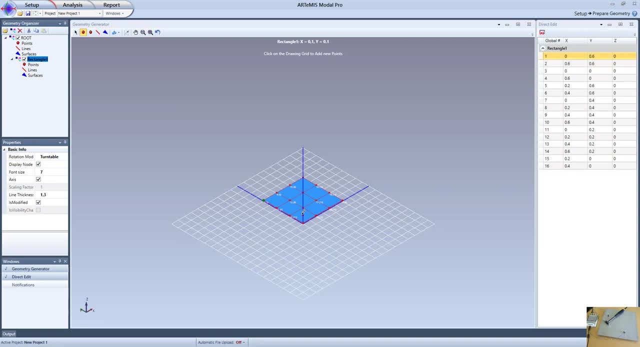 And now, I will then position the first one around this position here, And the second one will be over here, somewhere Like this: And now, that's it. I don't need to do more in this case. here I will go to the next task that I need to do. 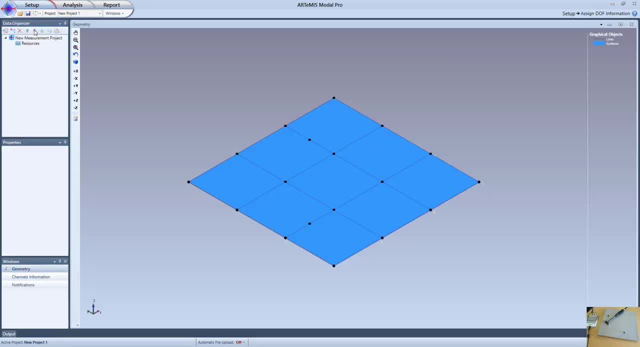 And that is the one where we define the sequence we are going to do the impacting in And with the number of sensors- input and output sensors- that are needed. So what I do now is I will simply select the top item here in the data organizer. 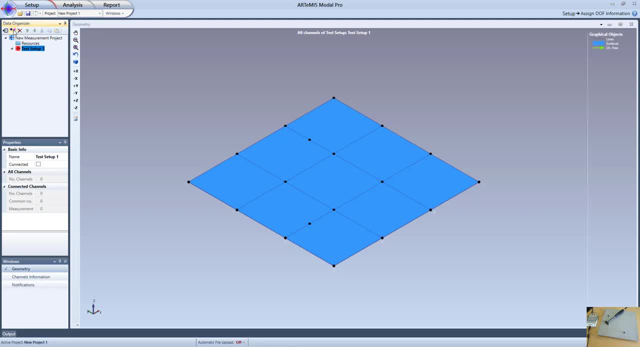 And I will insert a new test setup And insert three channels here. The first one here will be the impact hammer. As you can see, it's located here on the first channel, So I will simply inform Artemis that it's an input channel. 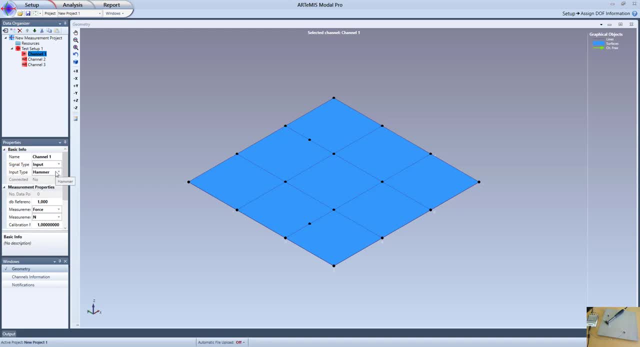 It automatically, By default, sets it to a hammer impact And then I will drag it out And then position it here on the first place. I like to impact And I will position it in the direction of the impact. So that's in minus Z. 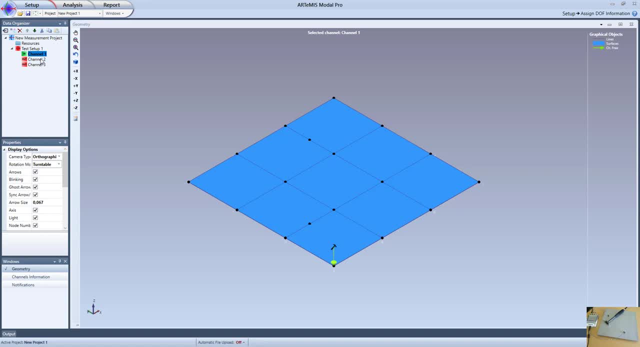 The next one, next accelerometer, will be the one located in this reference position here, And now it goes the other way, Plus Z is the direction for this one here, And finally we have the other one over here, also like this. So this is the first setup, the first impact position that we have defined here. 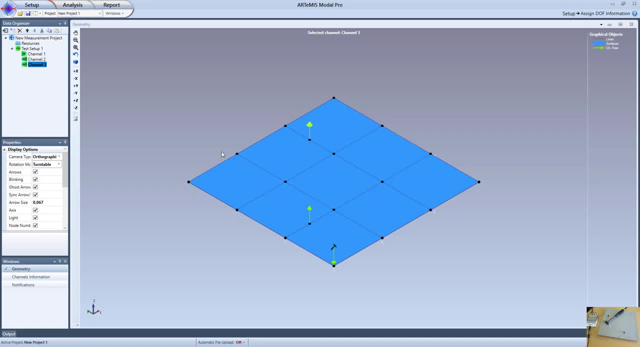 Now we need to replicate this. We need to do exactly the same for all the other points, And we have 15 points left that we need to impact also in order to get the mode shape of the full plate. So what I will do now is I will select this item here. 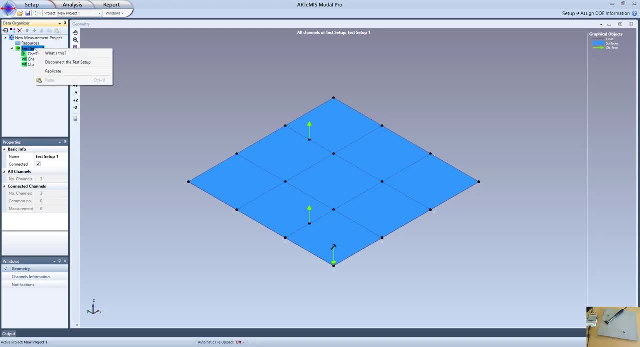 This setup item And then I will right click the mouse and choose this option here called replicate, And then I will tell Artemis that I need to replicate this 15 times And I also tell that I have two references here: The two output sensors. 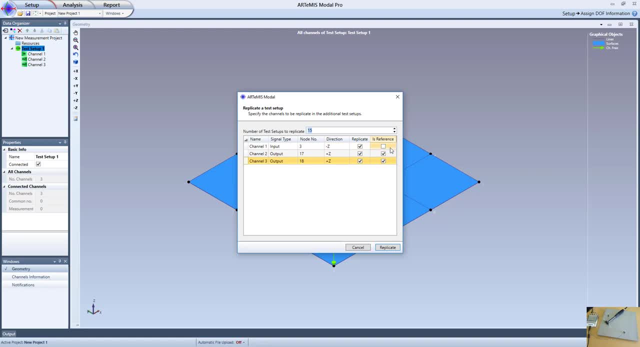 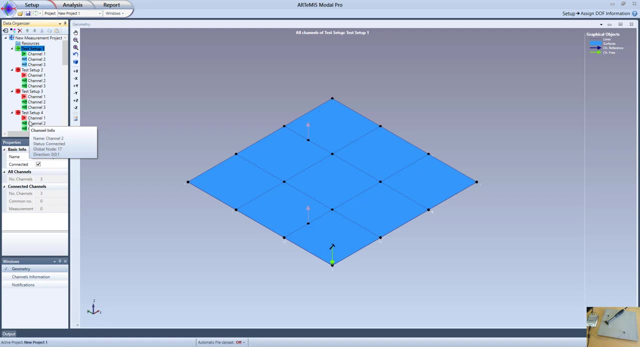 So the only one that I basically need to move to another position in the replicated setups will be the first channel with the input, And then I click the replicate button, And now we have additional 15 setups available here. So what I have to do now is simply to place this one here. 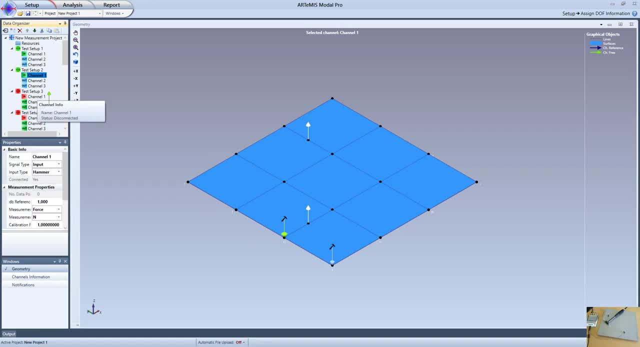 The impact position of second and to the 16th impact position. So I simply have to go all the way through here And drag these out And we have our first two, The first and to the 16th impact position And finally the rest. 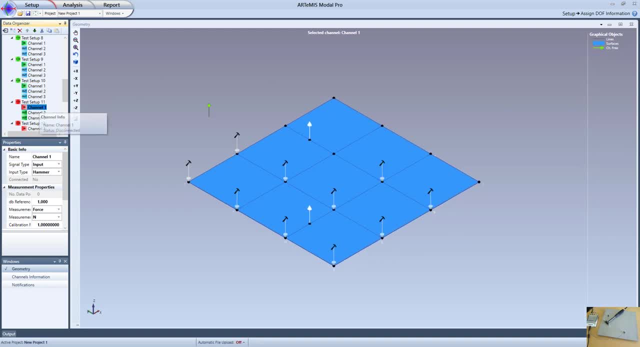 So I will exit this one here And go back and see where the first one was, And then I will drag back to the 14th impact position And I will click the same button and go to the last one And I will go back and see where the last one was. 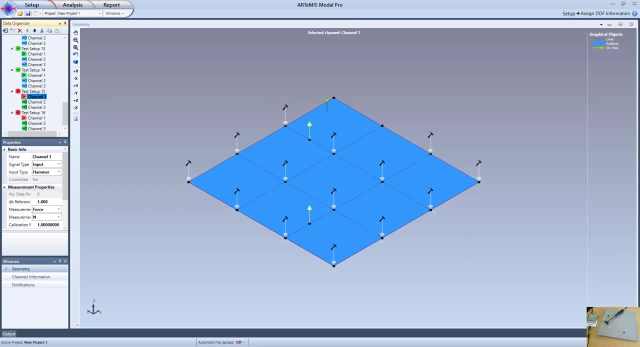 And I can also drag this one here And go ahead and open this one. And, finally, I have all the points that I'd like to impact marked on the plate here And we can see how Artemis automatically figured out that these are the two references.